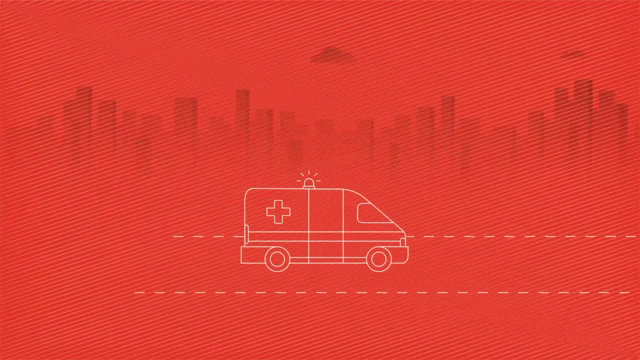 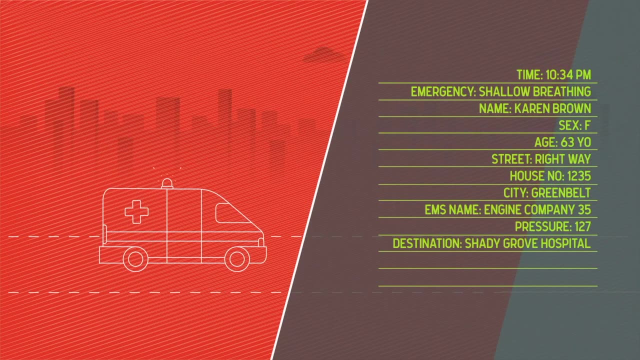 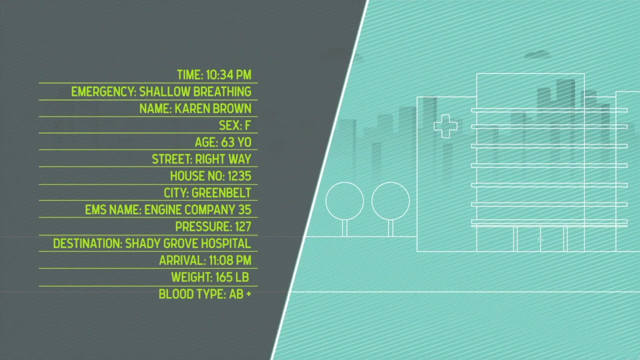 Okay, This is a typical call that 9-1-1 operators receive every single day. Each call provides a wealth of information about a person in need. In addition to contact information, EMS and hospital staff add health information to Karen's medical record as they treat her. 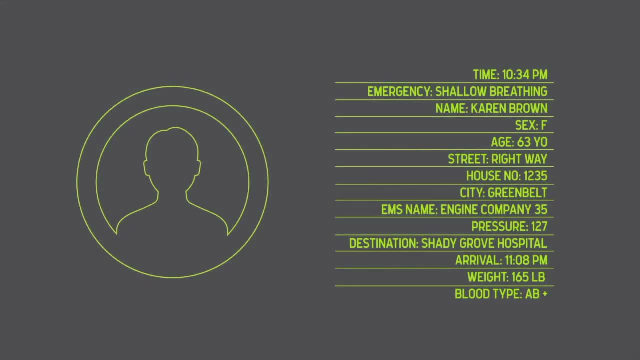 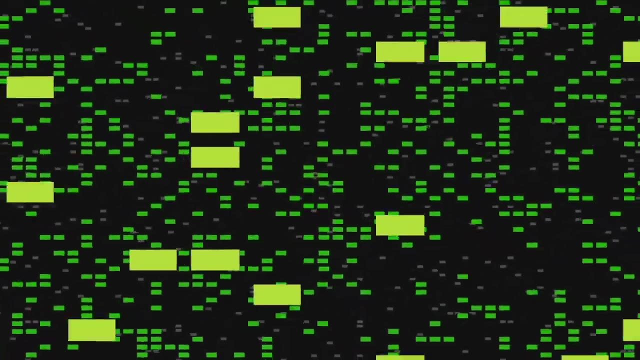 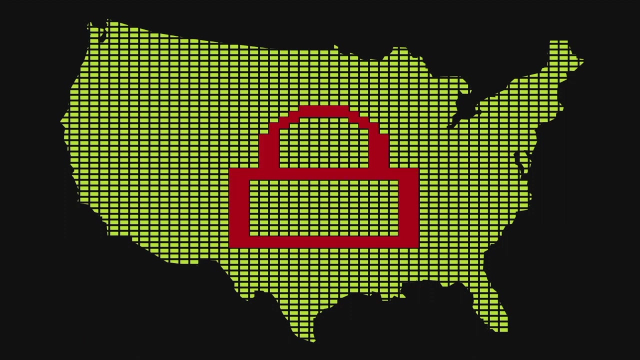 Most of this data is PII, or Personally Identifiable Information, which is key to a person's identity. This information is stored in large databases all across the country. Use of this data is protected by law in order to preserve your privacy. But what if we could use this data without compromising your privacy? 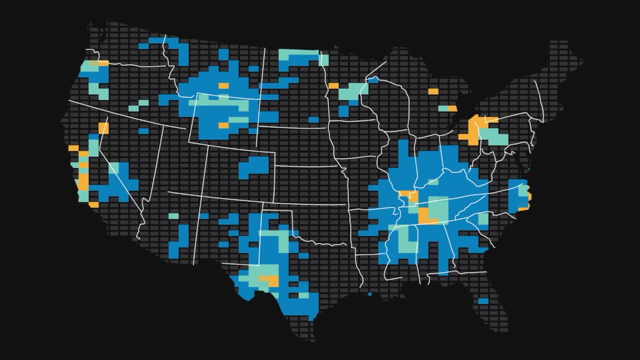 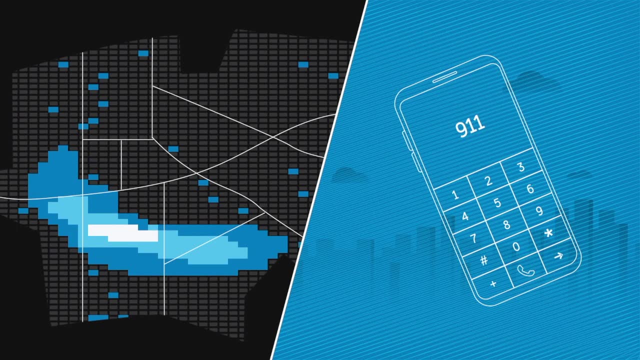 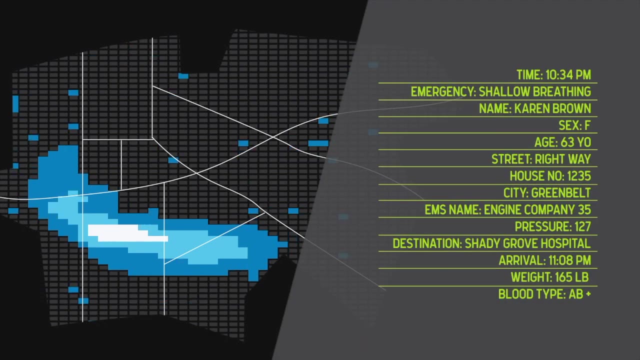 Imagine if we could aggregate data to see trends. What if access to Karen's and others' data show that 9-1-1 had received multiple calls about breathing problems around the same time? We might pinpoint the culprit Right now. use of data in this way is allowed as long as we redact the Personally Identifiable Information. 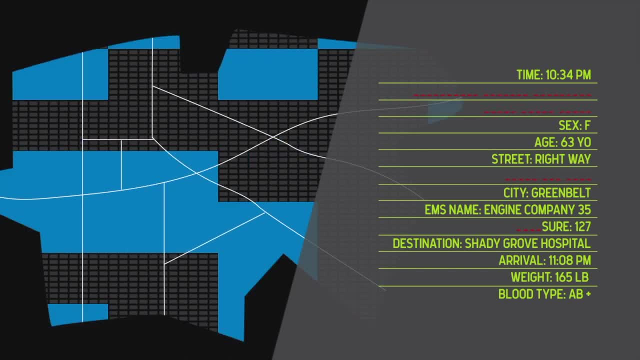 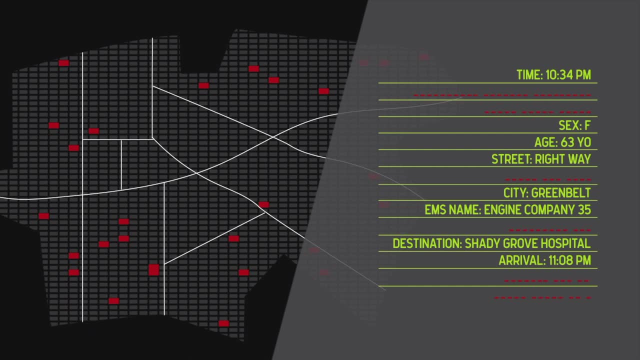 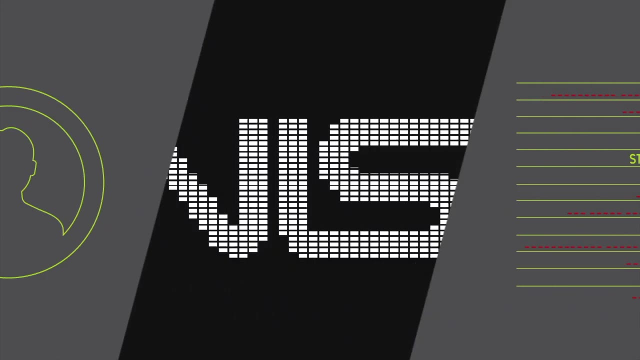 But by removing PII we drastically limit the data's usefulness and we don't always protect identities. For example, if Karen lived on a small street, her identity could easily be revealed just by sharing her age and street name. NIST scientists are seeking ways to improve the sharing of data while protecting individual identities through measurement and evaluation. 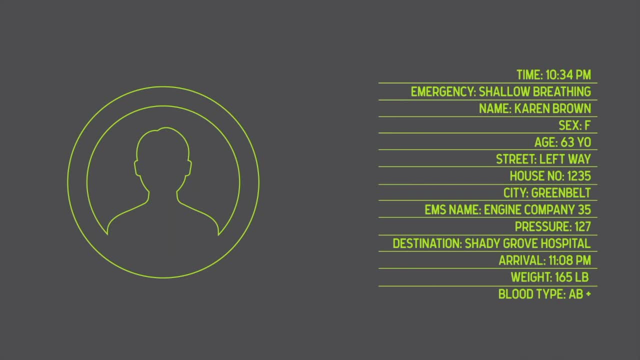 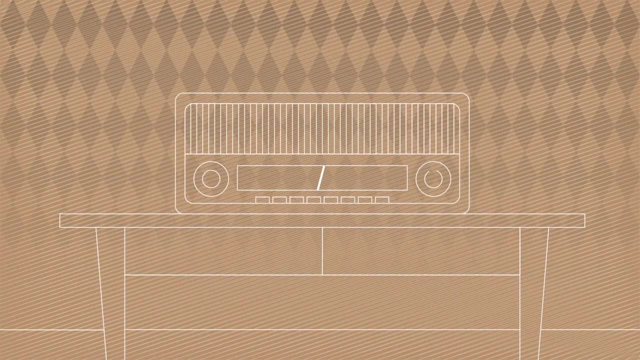 By slightly altering the personal information, for example Karen's age or home address, we reduce the risk of compromising privacy while still allowing data to be shared. Altering the data is like adding a bit of static noise to a radio broadcast. When your radio is tuned in to the exact frequency of the station, you clearly hear what's being said. 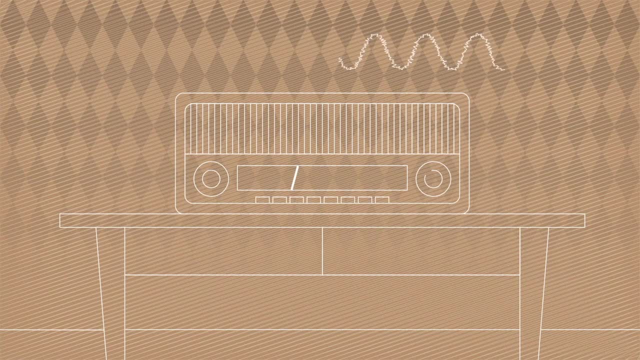 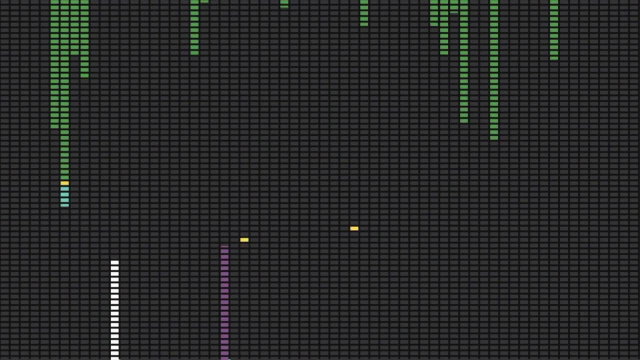 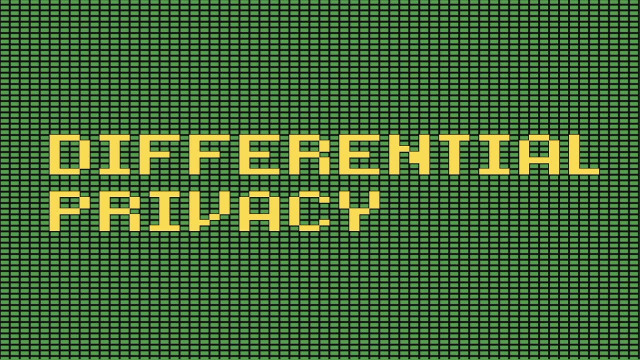 But if you move the frequency a bit to the left or right, static noise muddies the sound but doesn't compromise the message. This process of adding carefully tailored noise and altering identifiable information within whole datasets is called differential privacy. When this process is applied to large amounts of data, it becomes a provable guarantee of privacy.